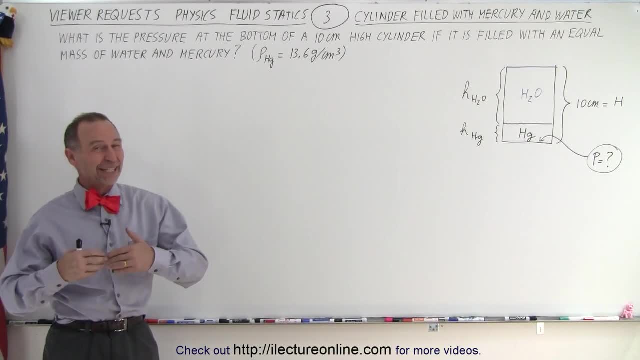 Welcome to iLecture Online. Here's another very interesting view request video. It has to do with a cylinder 10 centimeters tall and it's filled with a combination of mercury and water, and they want us to find the pressure at the bottom, and the constraint is that the amount of mass of water 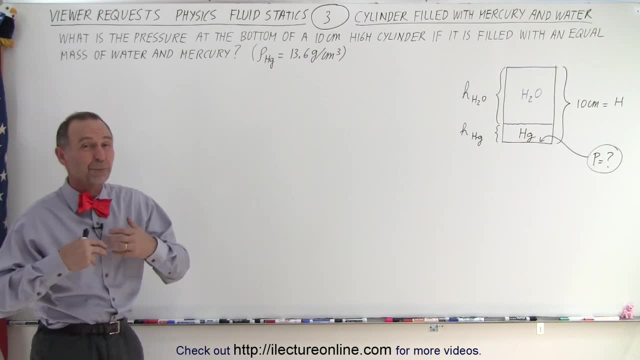 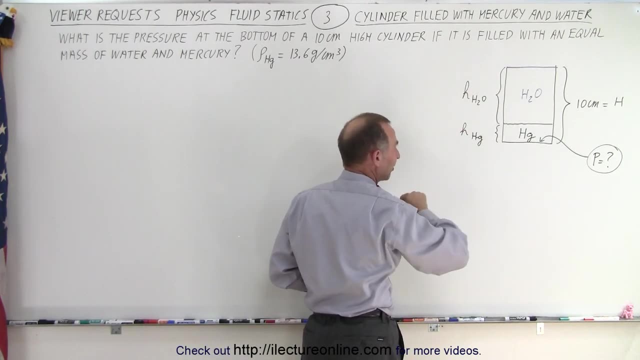 equals the amount of mass of mercury. Now, since mercury is a lot more dense, you would need a lot less volume of mercury compared to the water. The total height of the cylinder is 10 centimeters, so one of the things we're going to have to do is figure out what will be the height of the mercury. 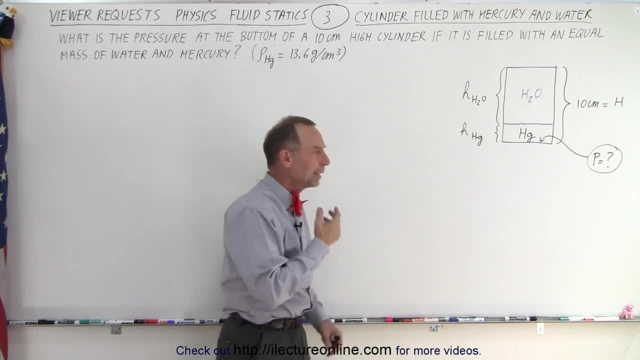 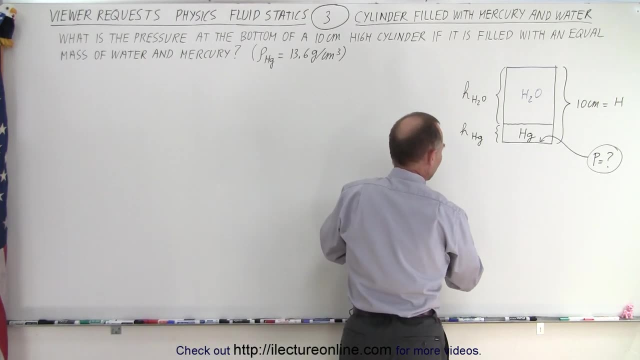 or the depth of the mercury and the depth of the water proportionally. So how do we do that? How do we figure out the pressure? Well, first of all, we have to understand that the pressure inside the liquid in general can be found by using the equation rho: g, h, h being the depth of the liquid. 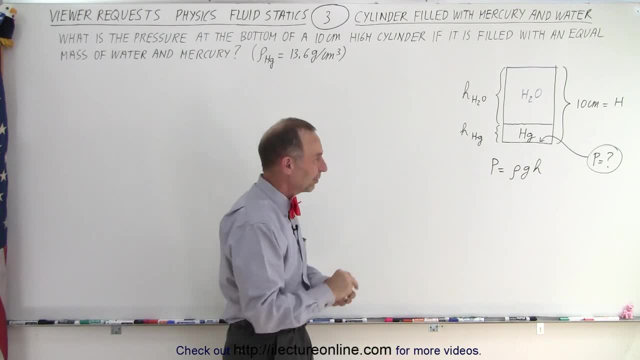 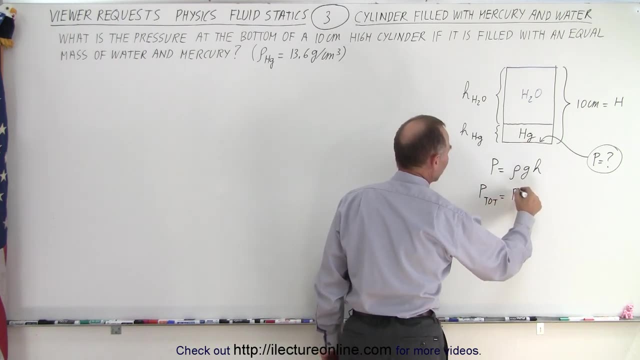 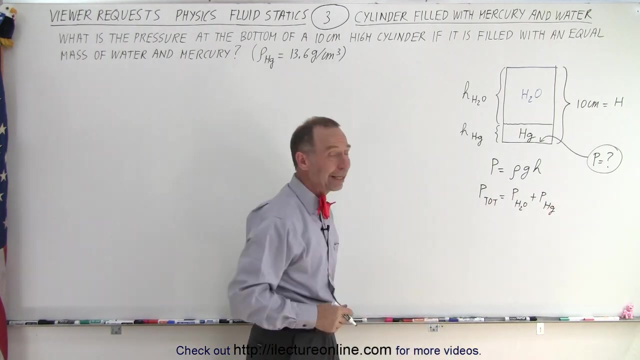 g the acceleration due to gravity, and the rho is the density of the liquid. But if there's two densities, we can say that the pressure total will be equal to the pressure of the water plus the pressure caused by the mercury. So we simply add the two together. Of course, what that means is that the 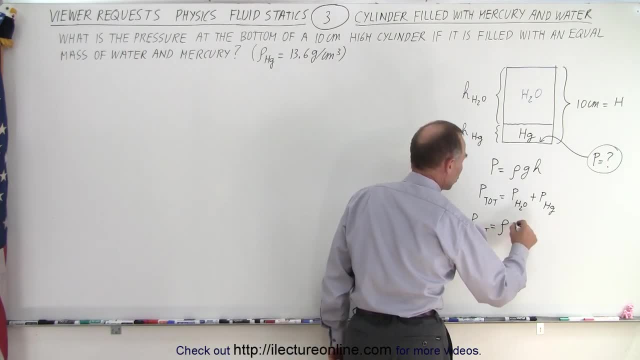 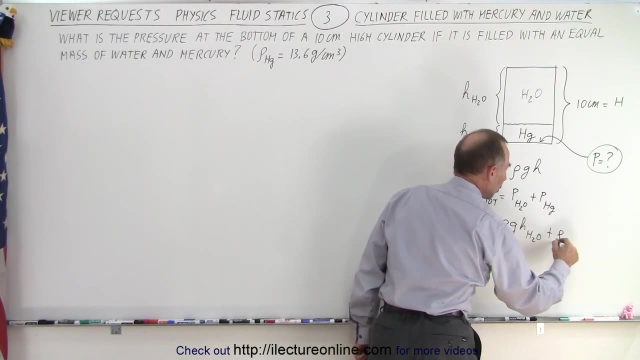 total pressure will be equal to the rho g h of the water. and notice this h of the water is this height right there, plus the rho g h of the mercury and of course this is the density of the water and this is the density of the mercury. Now we know the density of water is a thousand kilograms per cubic meter, or one gram. 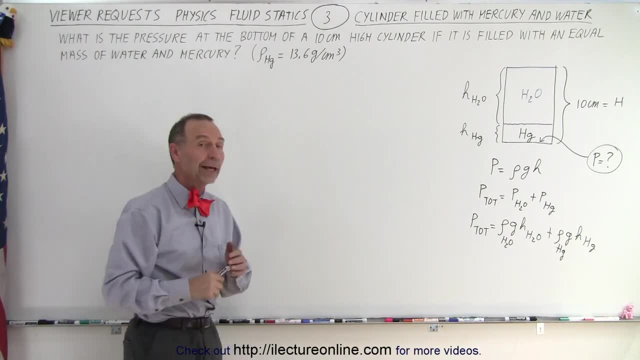 per cubic centimeter and the density for mercury. for those who don't know, that is 13.6 grams per cubic centimeter or 13,600 kilograms per cubic meter. So how do we solve this? Well, the key is that they tell us that the mass 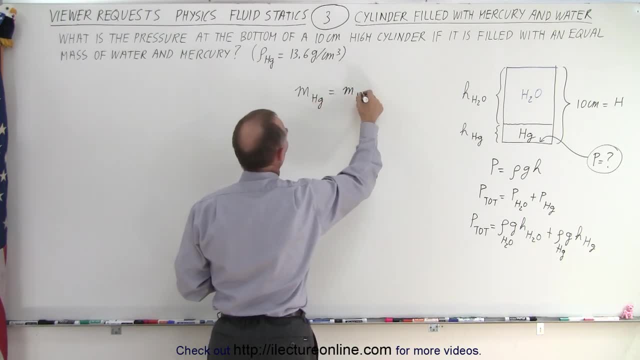 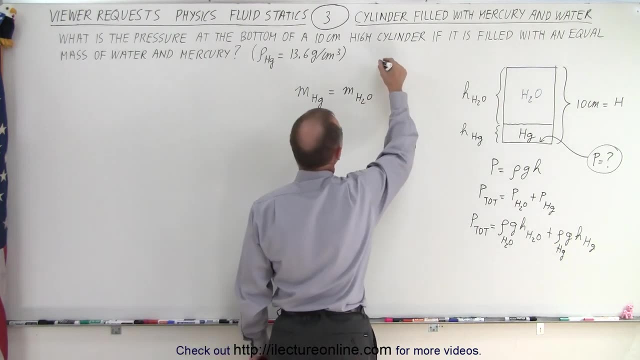 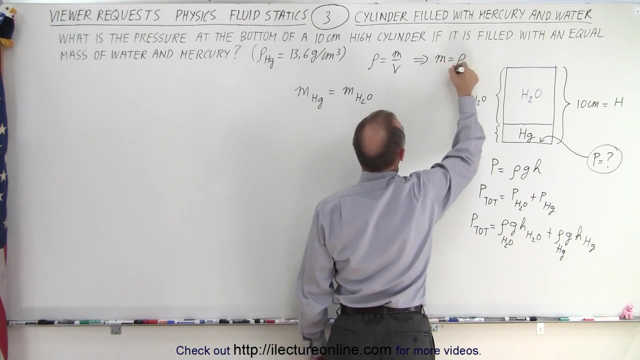 of the mercury equals the mass of the water. Now we have to relate the mass to the volume and the density. so what we can say here is that the density is equal to the mass divided by the volume, which then implies that the mass is equal to density. 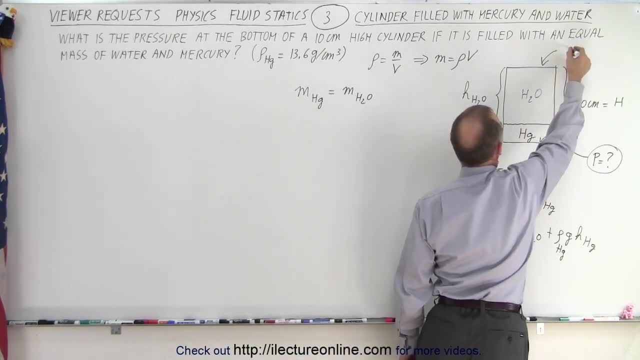 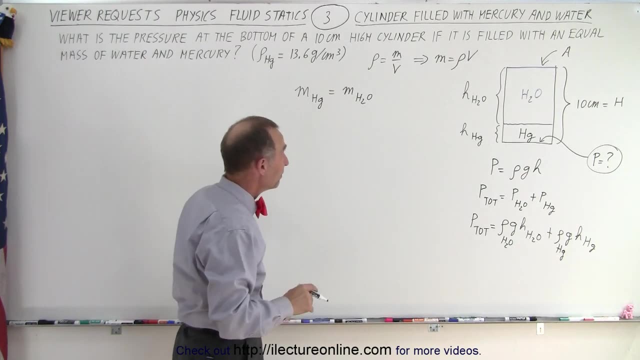 times the volume. Now, if this is the cross-sectional area and then this is the height, then we can relate the height and the cross-sectional area to the volume, and so we can replace these two M's by what they're equal to. so we could say that the density of the 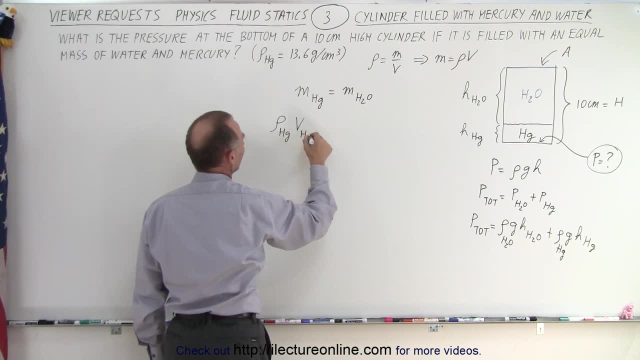 mercury times. the volume of the mercury must equal the density of the water times the volume of the water, and again the volume of a cylinder will be the area of the base times the height. so in this case that would be the density of the mercury. the volume would then be the area of the base area times the height. 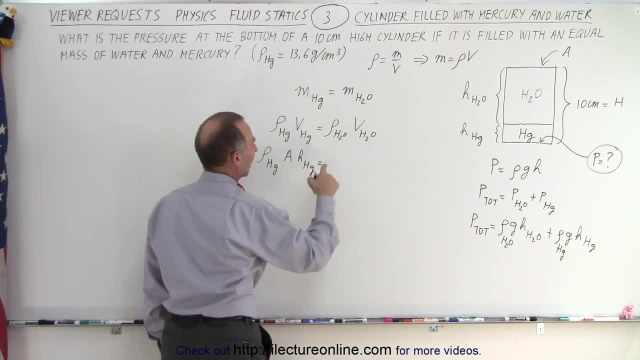 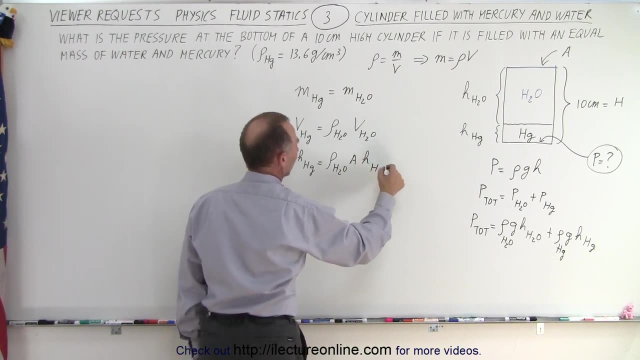 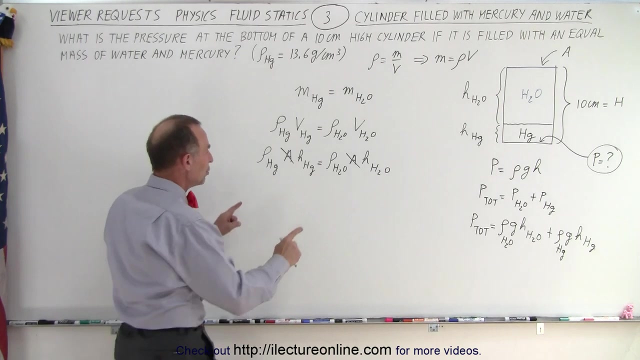 in this case the height of the mercury equals, and here we have the density of the water times the cross-section area, times the height of the water and notice that in both cases the area can cancel out because we have the same area on both sides. and now notice that we know the densities of water and mercury. so we 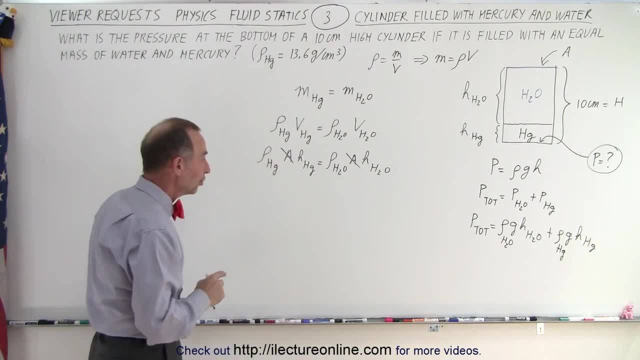 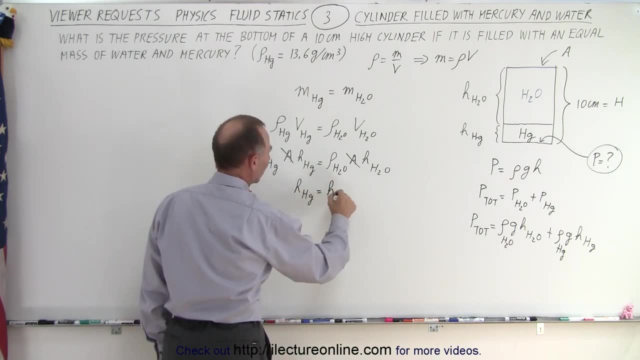 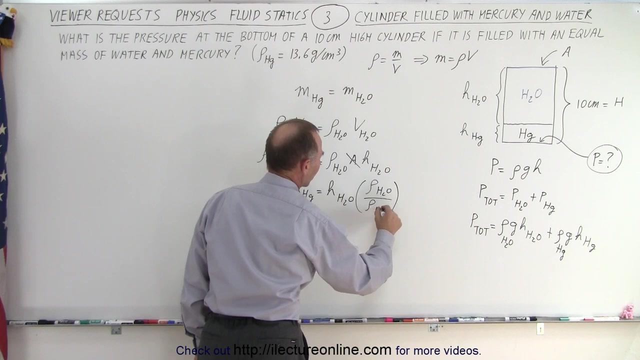 can find the ratio of the height of one and the other. so let's do that. we can say that the height of the mercury is equal to the height of the water times the ratio of the density of the water divided by the density of mercury and the ratio of that height of the 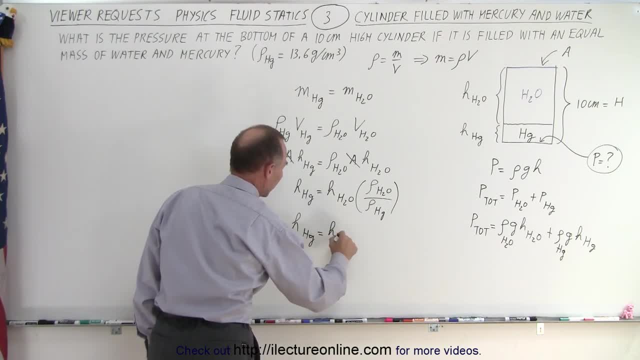 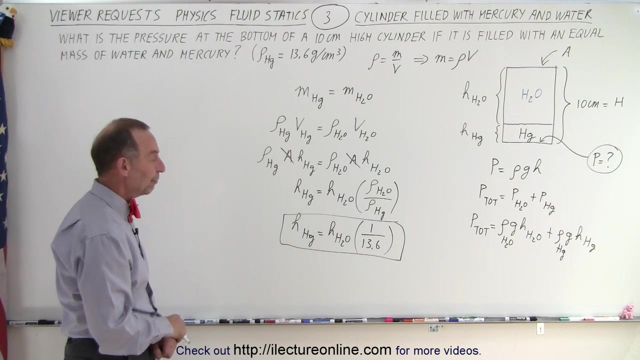 mercury is equal to the height of the water times the ratio of one gram per cubic centimeter divided by thirteen point six grams per cubic centimeter. so that's the ratio of the height of the mercury relative to the height of the water. now to find them. we realize that the two together add up to 10 centimeters. so know that the height 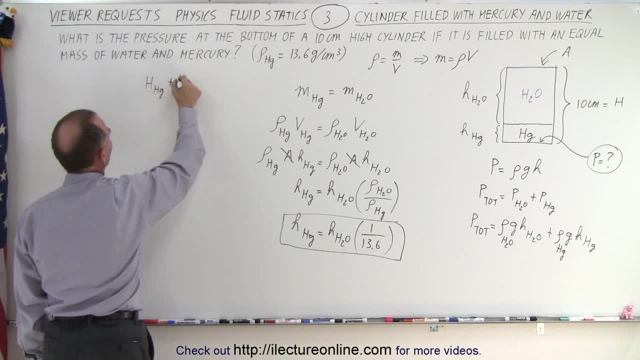 of mercury plus the height of the water equals, third, not 13, but 10 centimeters. and then we can replace the height of the mercury by what that's equal to. so we can say that the height of the water h2o, and I probably should have used small h's so we don't get confused here. go so the height. 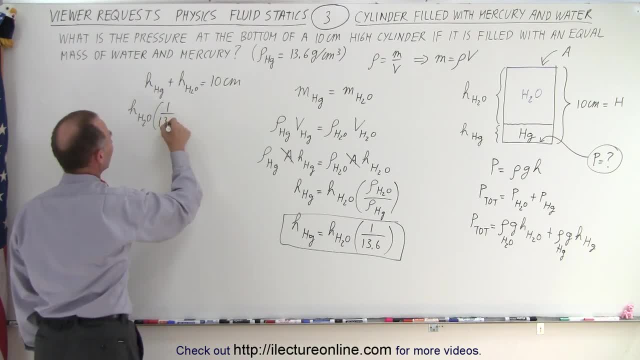 of the water times 1 over 13.6, plus the height of the water is equal to 10 centimeters. so now, when we add these two together, this is 13.6 over 13.6 plus 1, so we get 14.6 over 13.6 times the height. 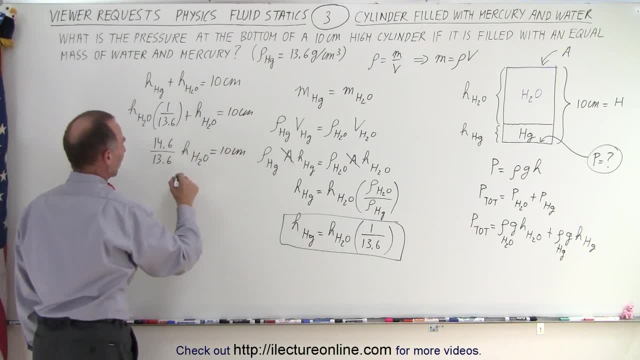 of the water equals 10 centimeters. so that means that the height of the water h2o is equal to 10 times 13.6. divided by 14.6 equals- there we go- 9.315 centimeters. so that's the height of the water. and now, by using: 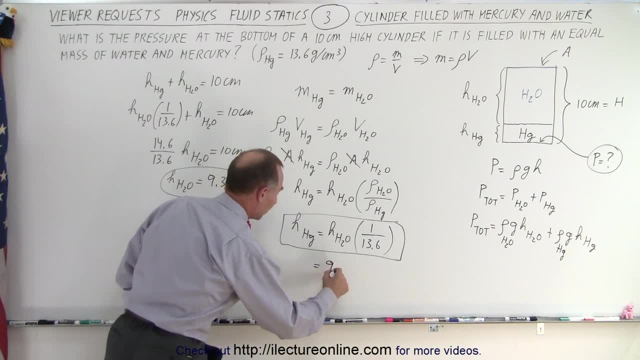 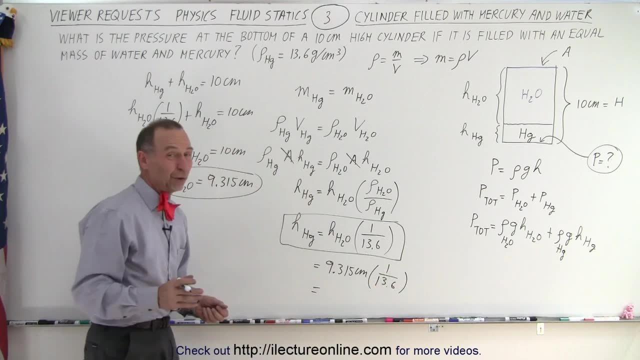 this. we can say that this is equal to 9.315 centimeters times the ratio 1 over 13.6. of course, we can say that this is equal to 9.315 centimeters times the ratio 1 over 13.6. of course, we can say: 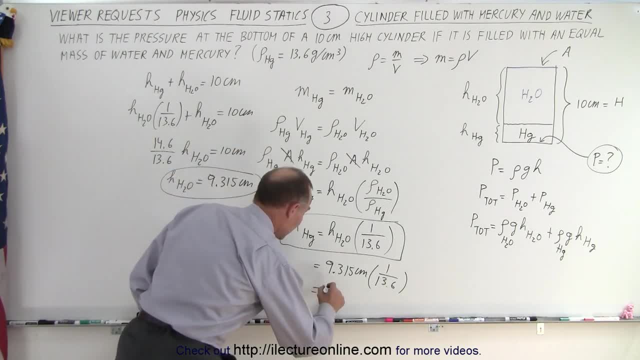 that this is equal to 9.315 centimeters times the ratio 1 over 13.6. of course, we can say also: subtract that from 10, and then the remainder would be 0 point. that would be 685 centimeters, and so that would be the height of the mercury. 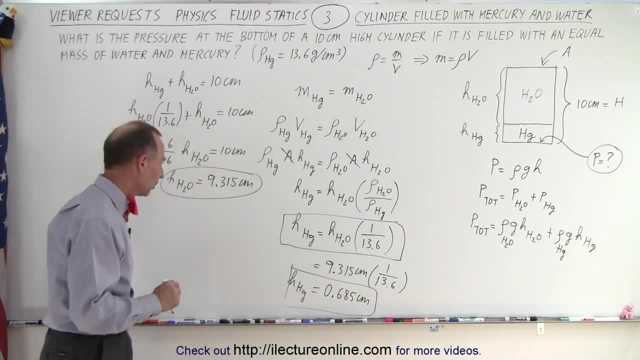 so we add this to this, that would be 10 centimeters. so we're good. so we have the height of the water, we have the height of the mercury. now we can find the total pressure, now that we know everything. so let's go over here and find the total pressure, pressure total. 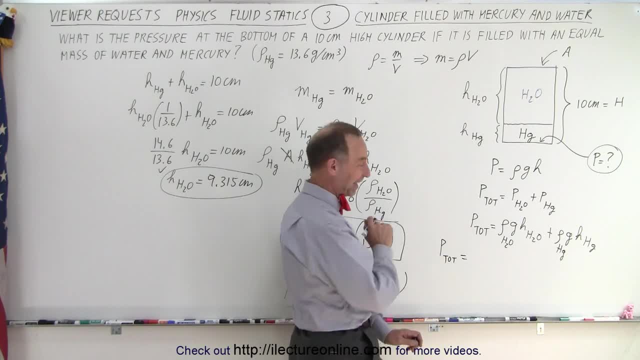 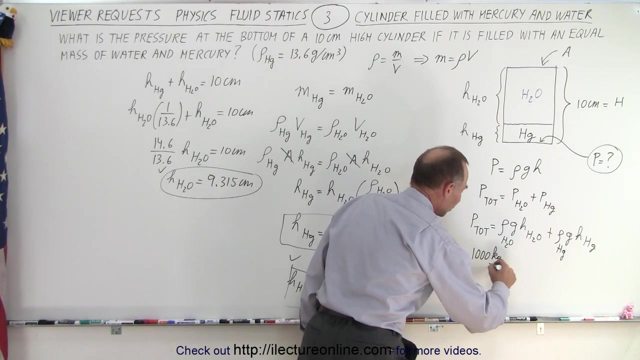 is equal to no, because i'm only doing that. the density of the water, let's see, we can do it in grams. now we'll do kilograms. that's better. density would be 1,000 kilograms per cubic meter. g: 9.8 meters per second square. 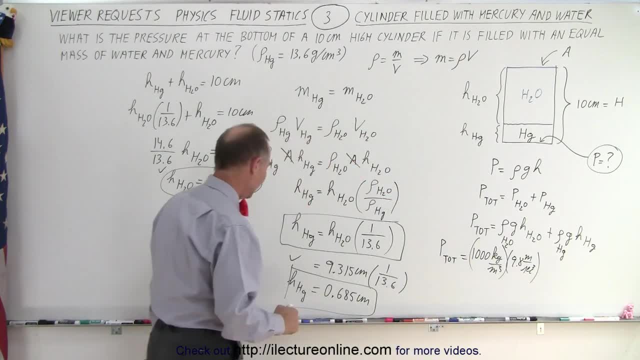 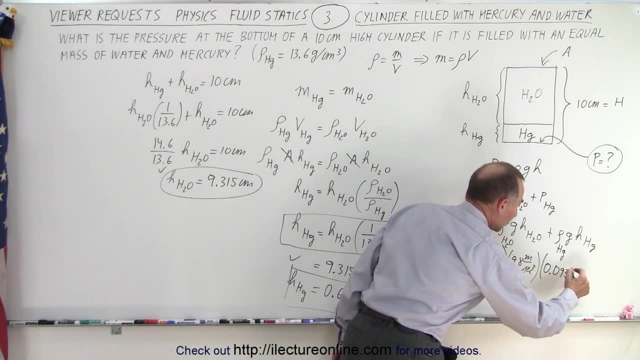 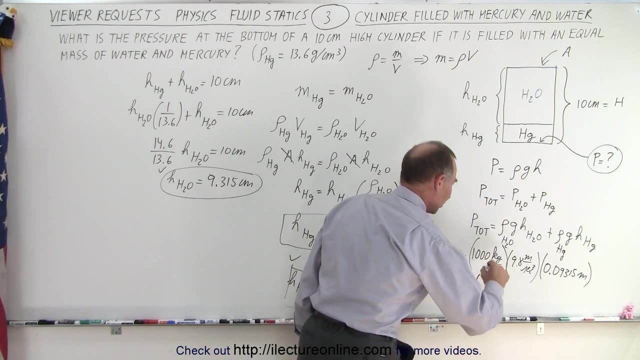 height of the water in meters- because now we're on convert out to meters- is equal to 2.5 impulses. the density of the water is 5.5 impulses ü now i can doкивuc attam others here- is equal to 0.09315 meters. that should be a five there. there we go, and then plus the density of 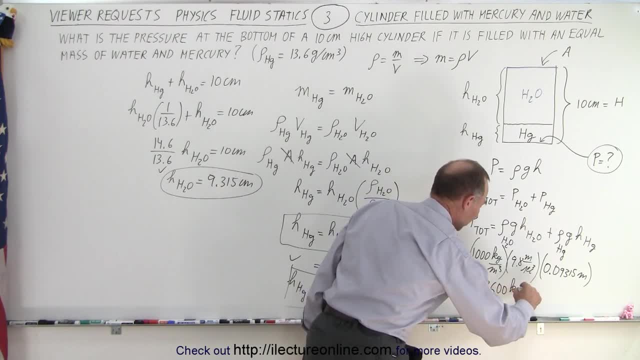 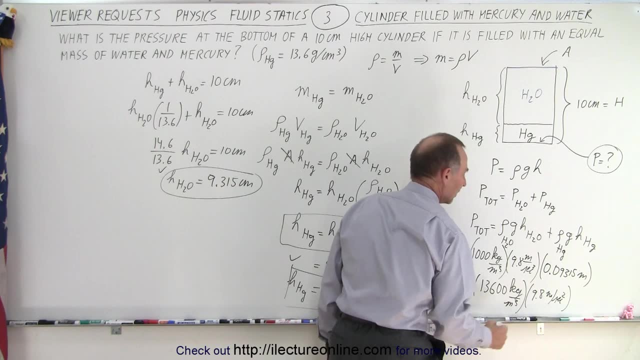 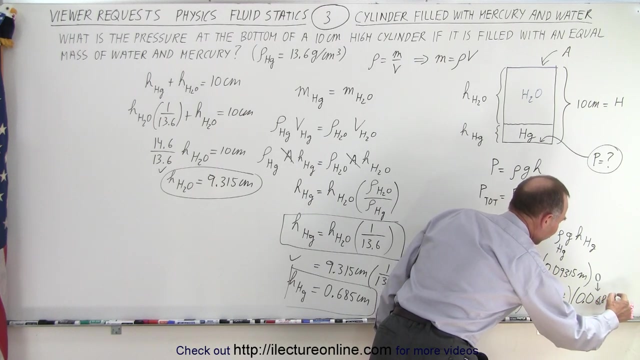 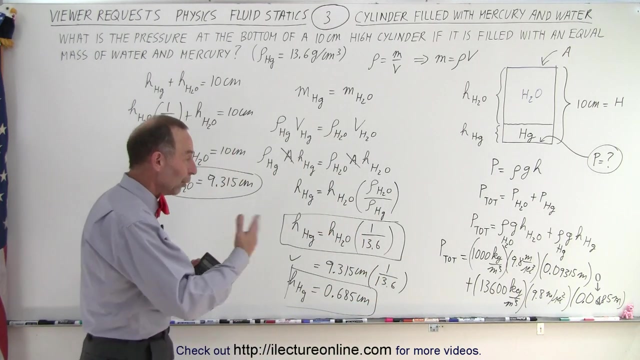 mercury: 13 600 kilograms per cubic meter, 9.8 meters per second squared and the height: 0.06 eight, five meters. okay, now, if we add those together, and you know what i'm going to do is i'm going to solve both of them together. i'm going to write each solution separately, because 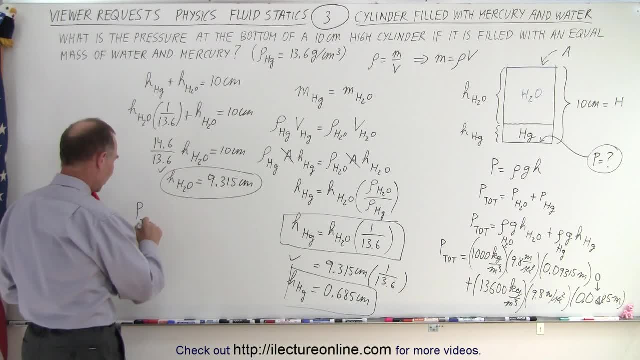 it's an interesting result because i worked it out in advance. so p total is equal to, so we have 9800 times 0.09315 equals, so we have rounded off 913 newtons for the pressure- oh, newtons per square meter, of course. 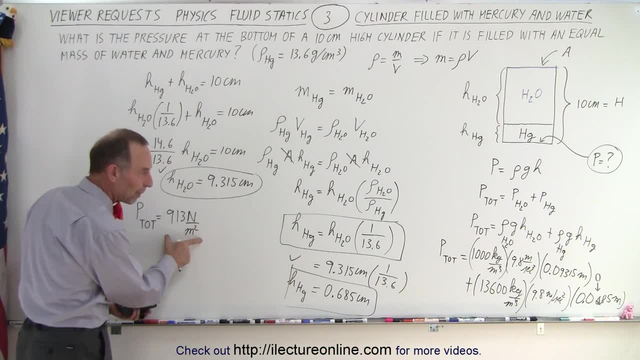 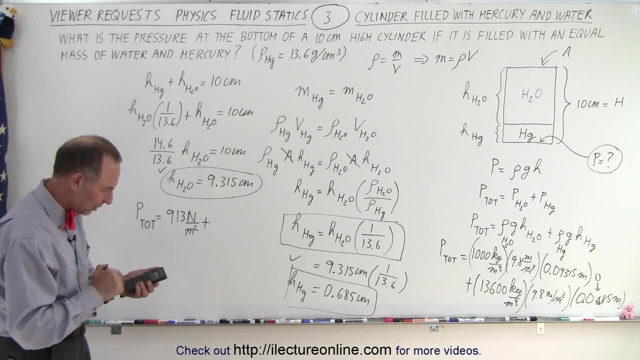 because it's pascals. so that would be the pressure caused by the water plus and the second one, that would be 13 600 times 9.8 times 0.0. am i missing a zero? aha, i'm missing a zero and the one more zero. in there there we go. one more zero, zero, zero. 685 equals and notice. 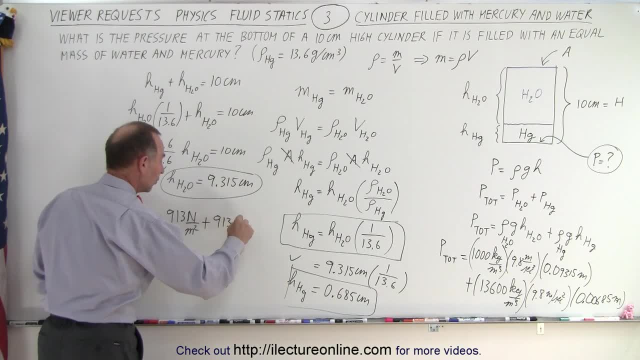 we get again 913 newtons per square meter and the. together that would be 1826 newtons per square meter for pressure total. but what is really interesting here is to note that the pressure applied by the water is not the pressure applied by the water, but the pressure applied by the water. 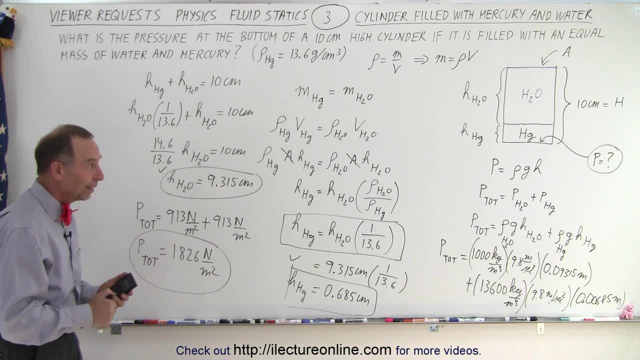 is equal to the pressure applied by the mercury. of course, the relative height depends upon their relative density. so the total weight, since the mass of each is the same, the total weight of each is the same and therefore the pressure applied by each is the same, and that's an. 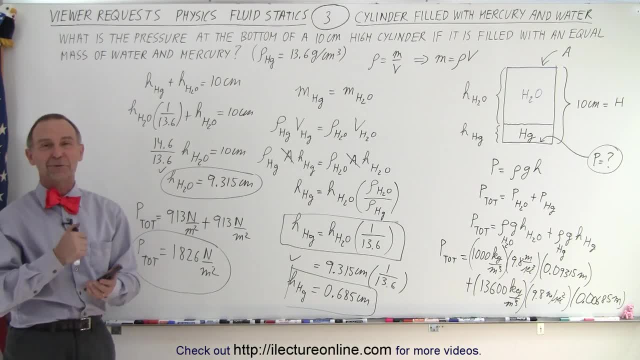 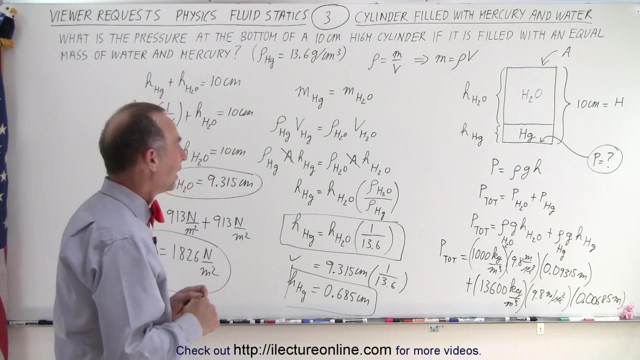 interesting result, and this is the answer. that's how it's done. you like classic problem? yes, it certainly is, but it was an interesting problem while we're doing so. the pressure of the water before it gets to the mercury is nine point nine hundred and thirteen meters, correct. so the pressure at this location